through the soil, that value increases to maybe double that through a larger plant. So having spring compaction is really detrimental to crops and that early rooting will set the stage for the yield potential throughout the year. Well, we know what it is. we know what it can do. how do we prevent it? 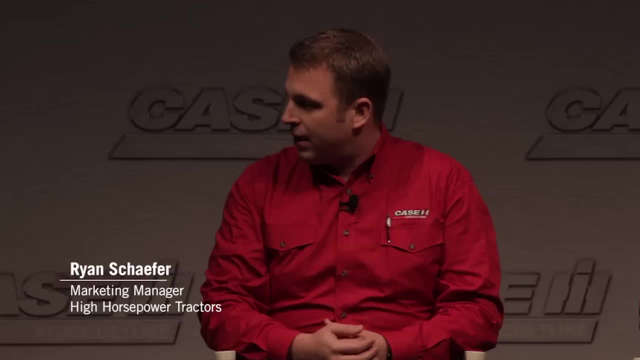 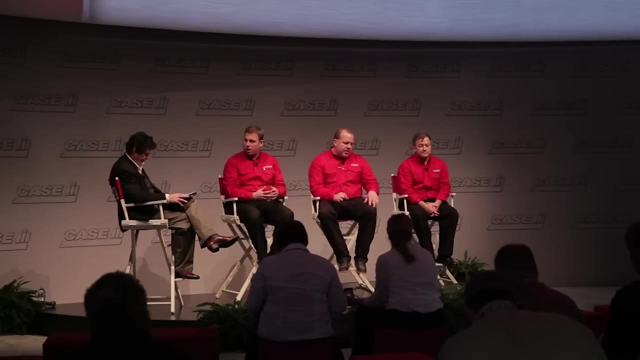 It all starts in the spring. It starts when you hit the soil that very first day with your seed bed preparations. There's other contributors as well. Rob identifies with seed trench compaction and early spring compaction as one of the greatest challenges we face as producers to try to eliminate. 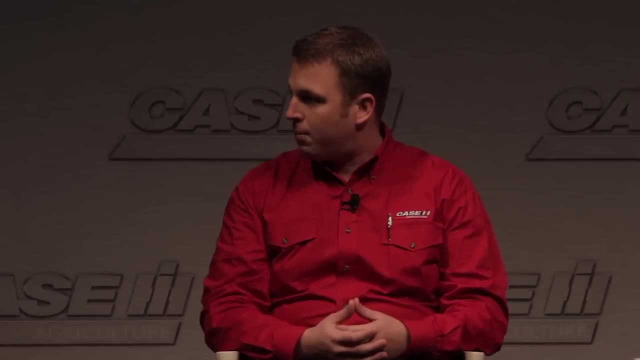 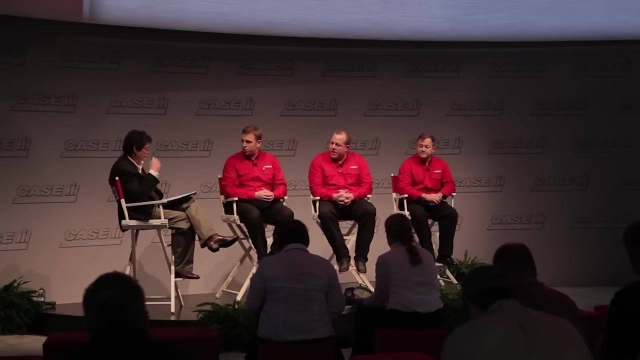 We want to provide a supple quality environment for that seed to start its growth stages in. We want to give the seed every opportunity to get off to a quick start, an early emergence with lots of vigor to create an opportunity for higher yield potential down the road. and 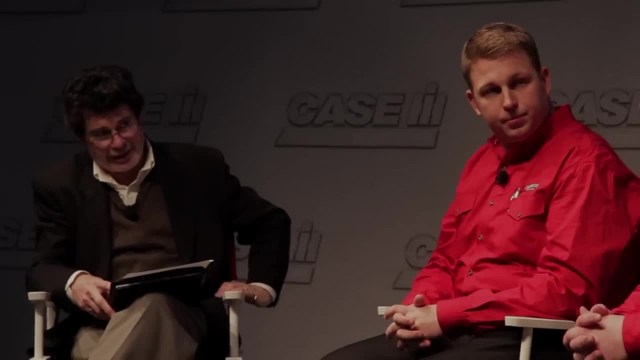 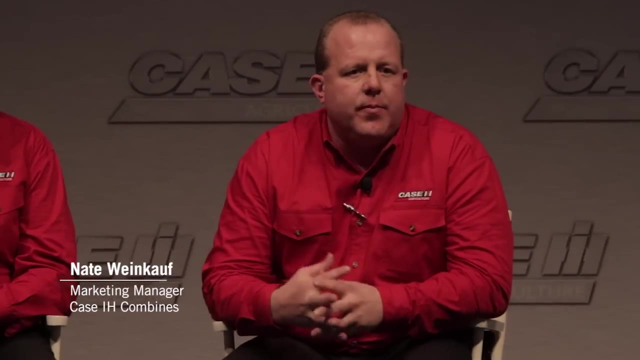 ultimately higher return on investment. Nate. I know combines have something to do with compaction. What has happened? our producers are continuing to add more acres to their operation. now They're traveling further, so they want to be more productive, more efficient. 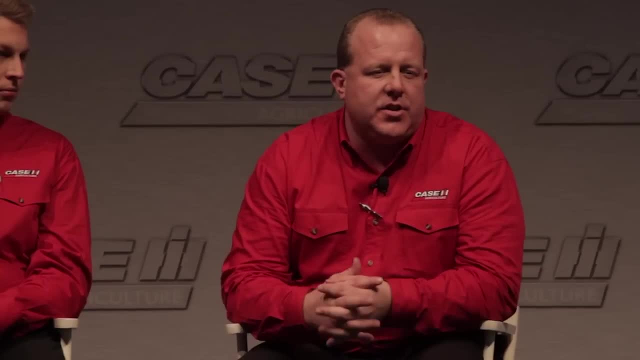 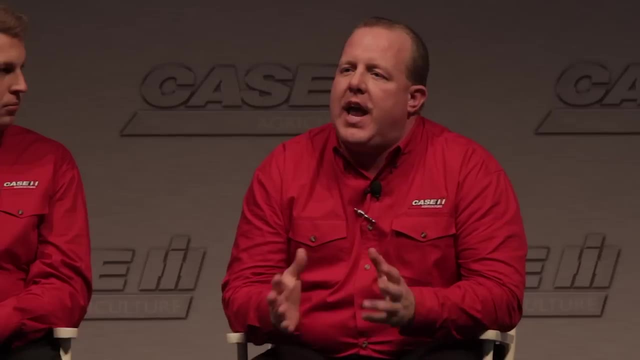 So now we're seeing, you know, class eight, nine, ten machines that are coming in and they're going to be more productive, more efficient. So what is that going to do? As we continue to go up in weight or up in class size, we're going to add weight. 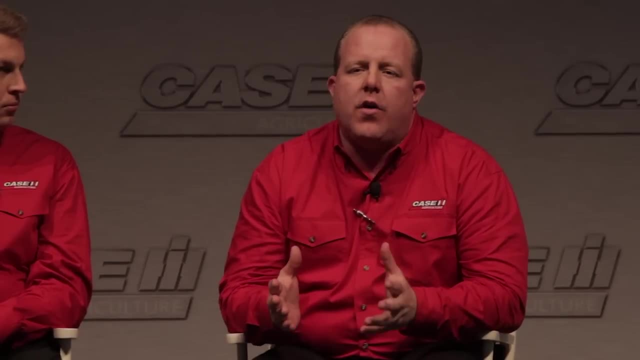 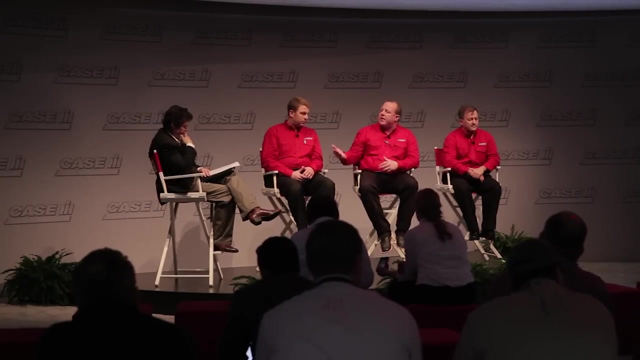 Being able to get out into that field. you know their harvest window. if they're farming eight, ten thousand acres, they're going to start at a certain time and they're going to have to go. So, getting back to talking about the track importance of it, that was something that we introduced here about three, four years ago. We haven't seen it, haven't had to worry about it too much the last couple years, but that fall of 2010,. really, across the majority of the area, We saw a pretty wet fall. 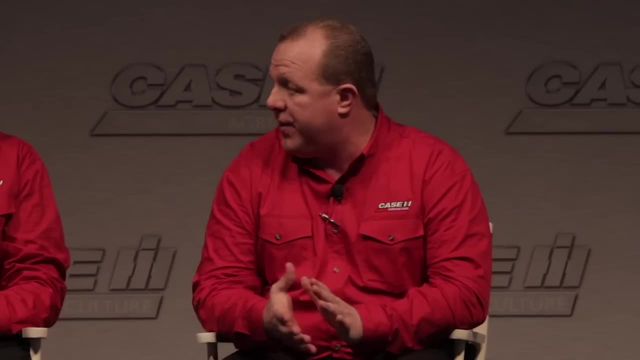 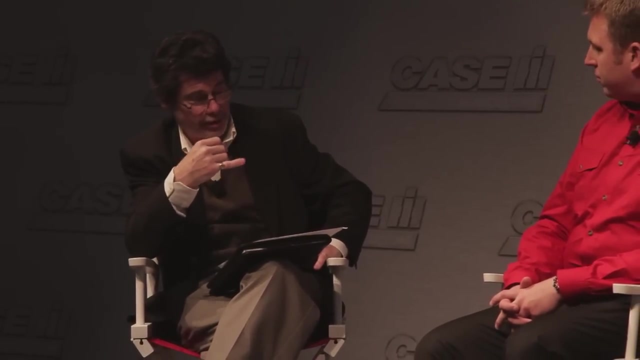 And with the track capability, customers were able to get their harvest, their crop, out of the ground. One of the key phrases we hear a lot about, and I know you've probably touched on this already, but when you talk about axle load, could you explain that in its relation? 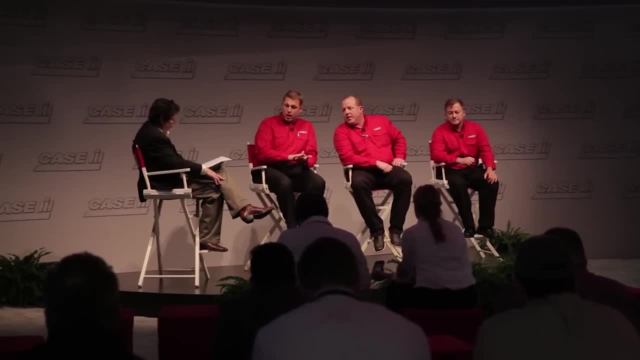 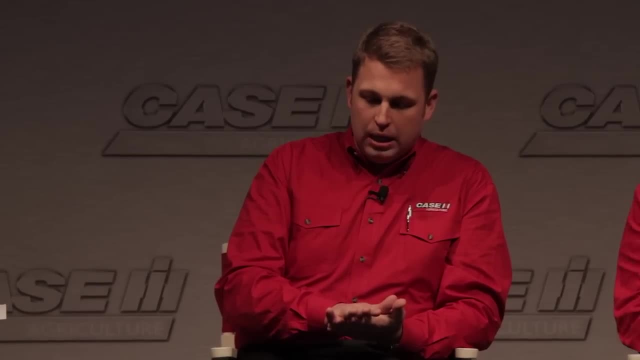 Ryan, We talk about axle load in terms of, and really total load on the soil in terms of pounds per square inch, I'm sorry. And when you look at it specifically, Specifically at the quad track design, you know we often talk about the agronomic superiority. 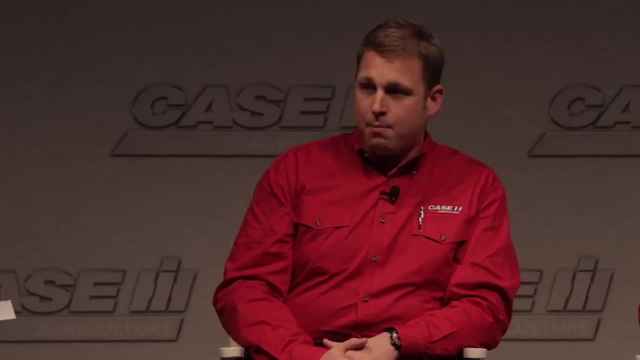 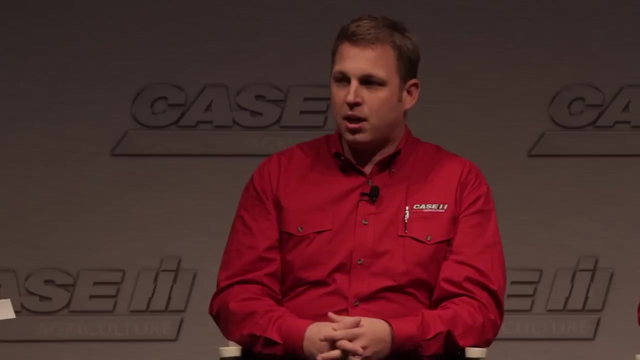 of the quad track undercarriage. It's why we've implemented it on our combine product. it's why we've gone to market with a newly developed row cropped offering with that quad track design, Because what the quad track allows you to do is equal out your axle load from the front. 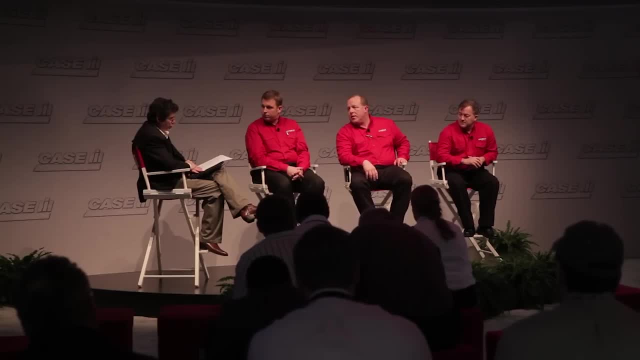 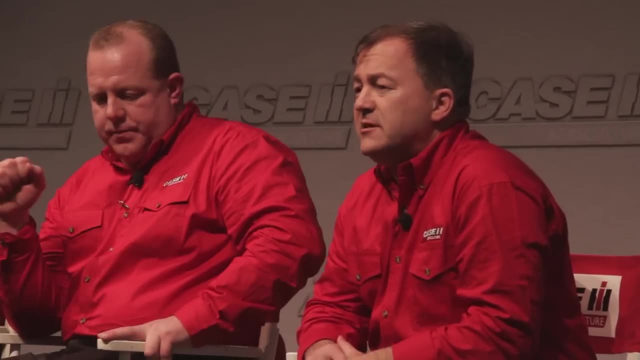 axle to the rear axle. Rob, do you have any other insights here? Yeah, sure, Jim, One of the great promises of tracks When they were first introduced into the- at least the rubberized tracks in the marketplaces- that we would make great strides in soil compaction mitigation. 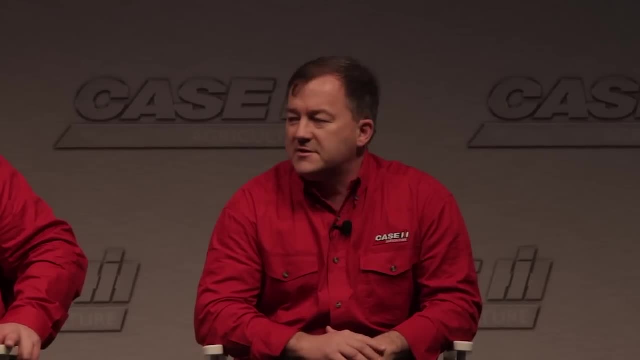 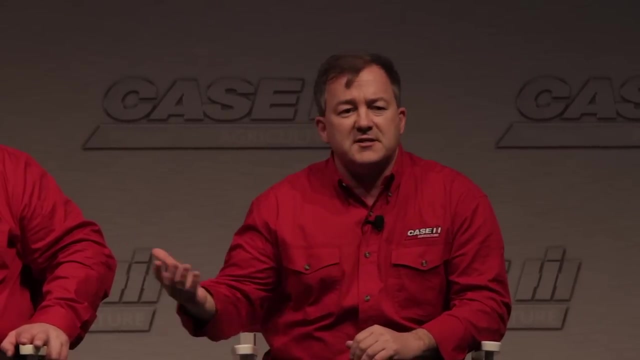 But I think the guidance systems had to come along to give us that repeatability so that year to year or season to season, we'd take full advantage of them, along with the balanced designs that have been mentioned here and the repeatability of our advanced farming. 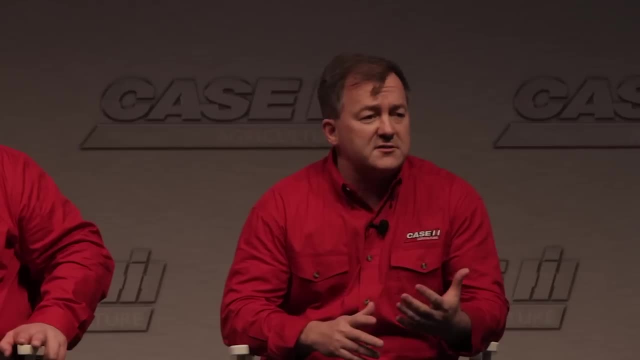 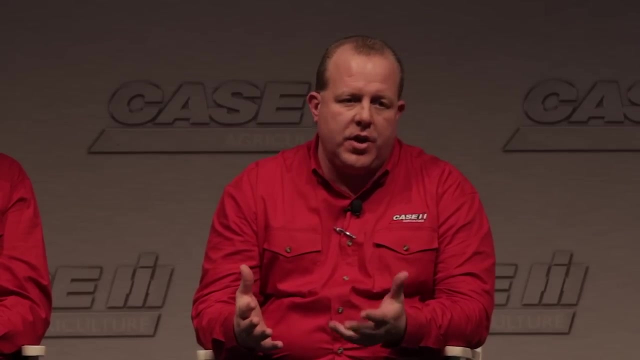 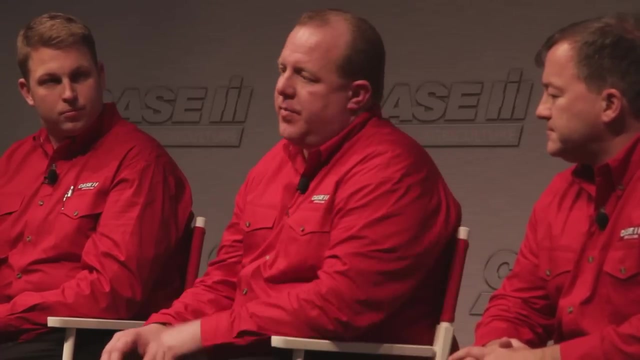 systems. That goes hat in hand with the ever increasing populations that we're seeing Corn production. today we talked about scouting and utilizing that information that you get from harvest season, with your yield and moisture maps, and being able to take those tools and work and go out and scout your fields to make sure that we're doing the justice and making 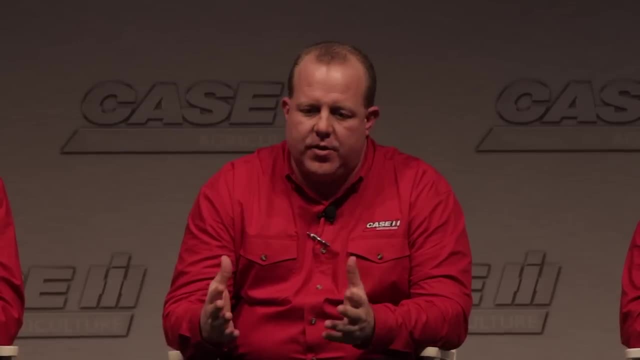 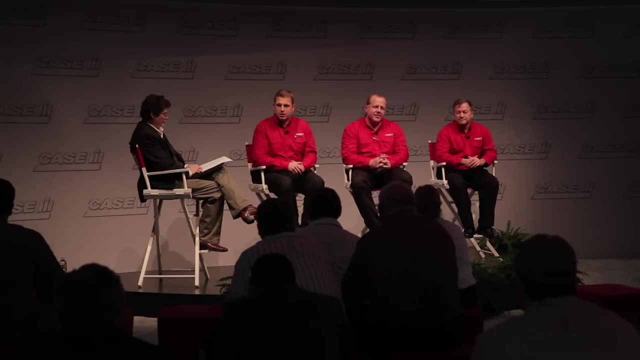 sure that we're achieving the most agronomic design or ability of that soil, of that ground, year to year, that we possibly can. Temporary compaction is likely a necessary evil, but I think the one thing we've learned as producers Is that it's a risk. 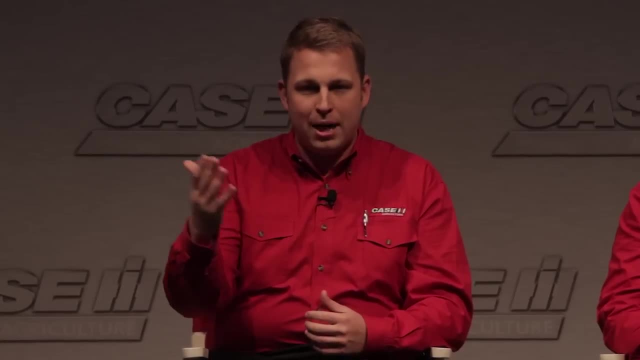 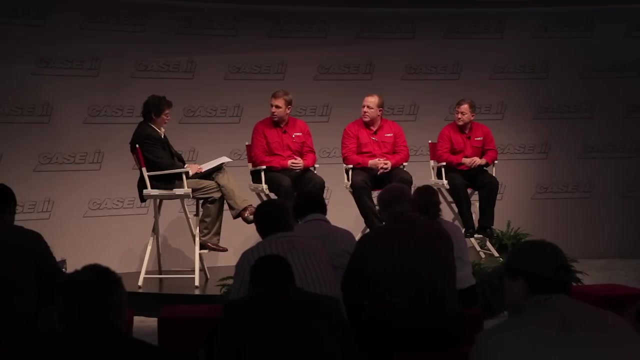 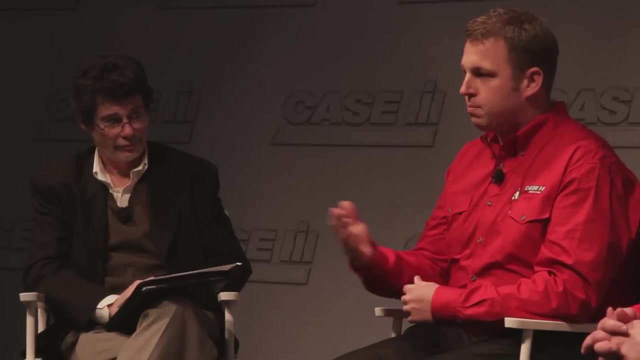 Like any other risk, whether commodity price risk or weather disaster risk, we as producers have options to be able to mitigate that risk. We have options through the choices we make, the implements and the farming practices that we choose to use and those business partners that we choose to do business with as an operator. 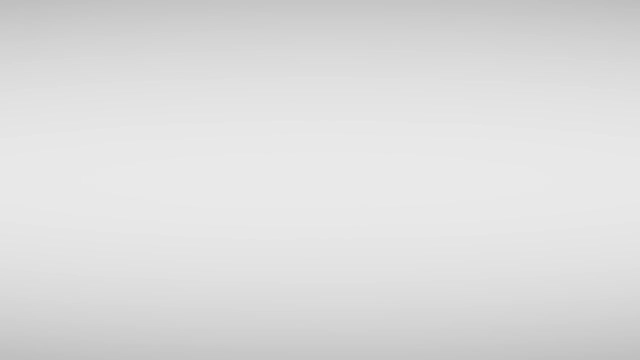 or who we choose to support us as a producer and as a grower. So I think that's a number one thing you need to think about for yourself as you're doing business. So, if I can just take a moment here and make sure that I'm sure my points are correct, all that I'm doing is I'm doing business in a way that's useful, and I'm doing it for our community and for the power of our ability to serve our communities. So keep that in mind, Thanks, Bye.